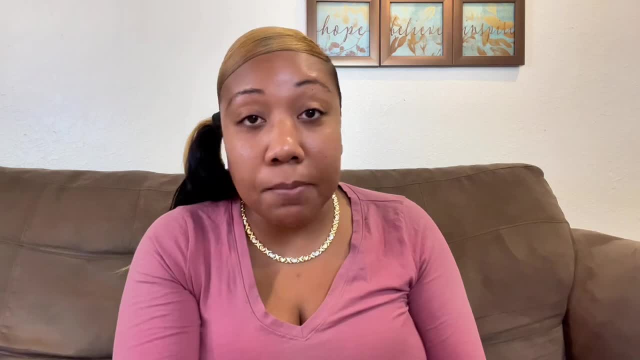 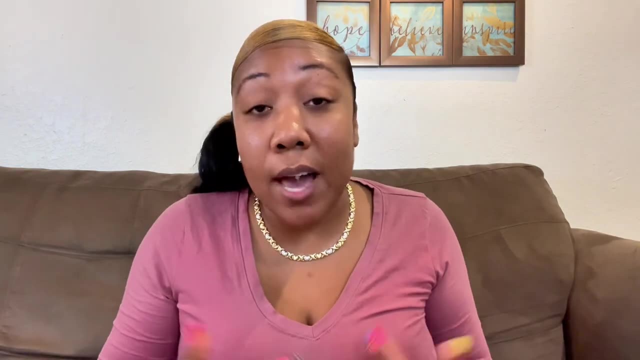 might be behind for a few weeks or so and you might have to pay interest, but you still can come up with a solution now to fix that problem. hey, if your phone bills due and you don't have the money, then you might have to be without the phone for a few days. i mean all of these issues. 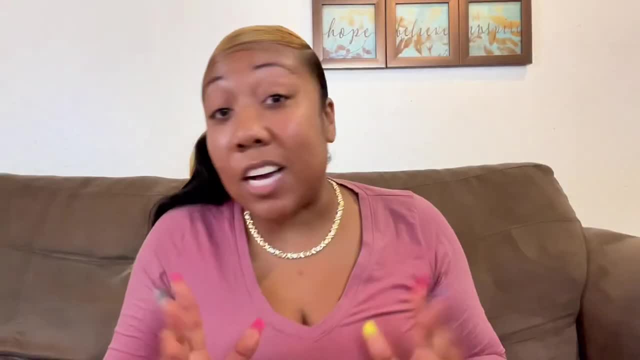 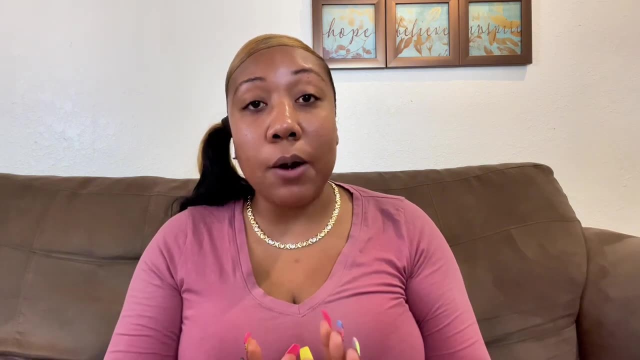 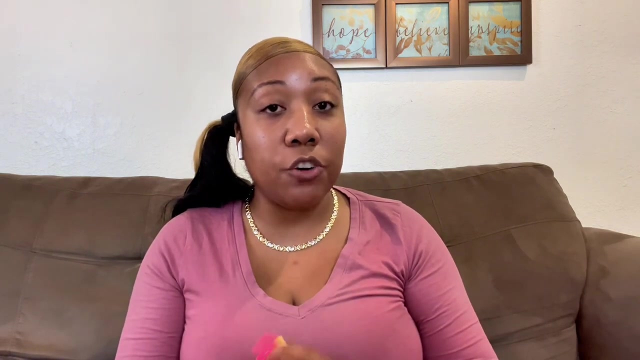 are just temporary, you know, as long as you come up with a solution. now, sometimes it's not that easy to come up with a solution, so what i do is sometimes i would have to just take a step back and view the situation. i remove myself and anyone that i know from that situation. 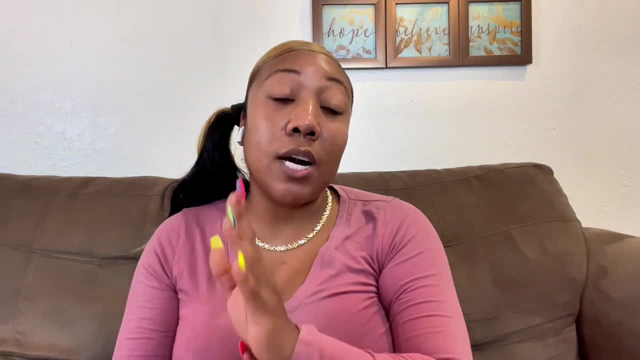 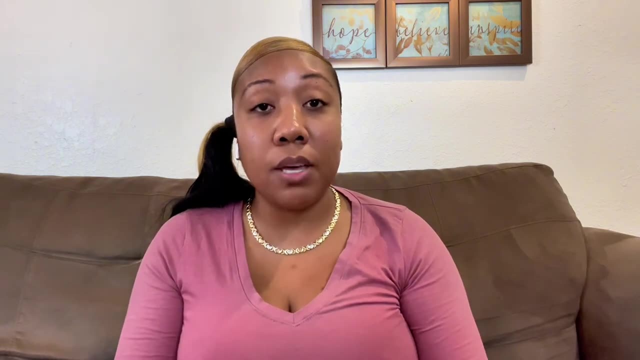 i will sit there and i will put your other people going through that same issue you, so that i can get a different perspective. that way your feelings will not be evolved. there might be a small amount of problems that you cannot fix. the one problem that i know. 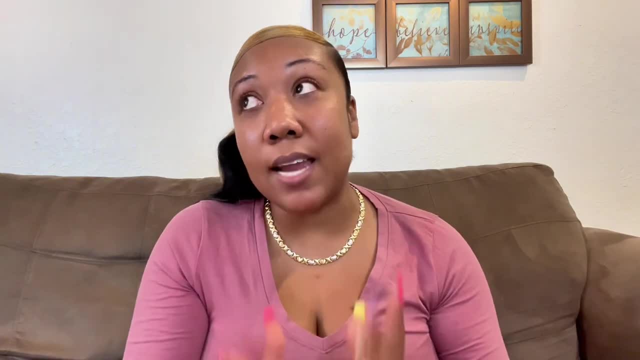 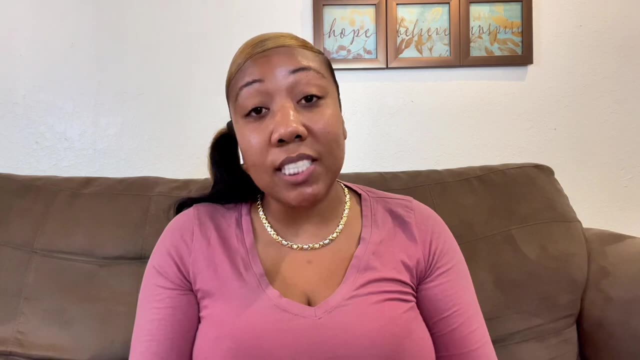 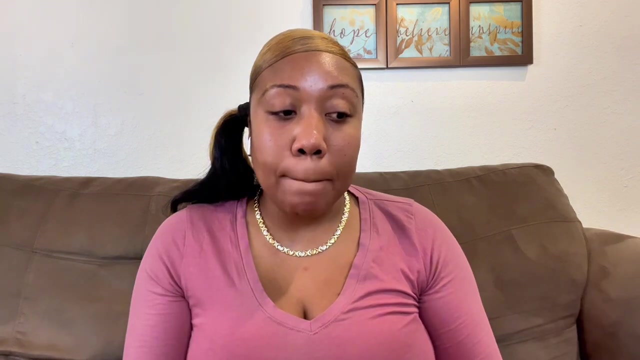 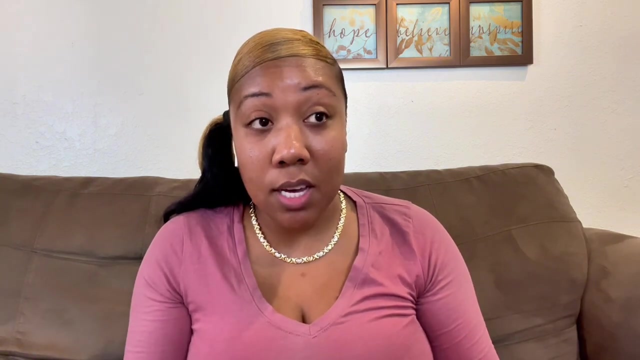 is dealing with grief. it's like you cannot fix that issue. you cannot fix something that happened that you had no control over. the only thing that you can really do in a situation like that is just to change your viewpoint on life in general. um, if you believe that there is so much more to life than this life here on earth, then you know you'll. 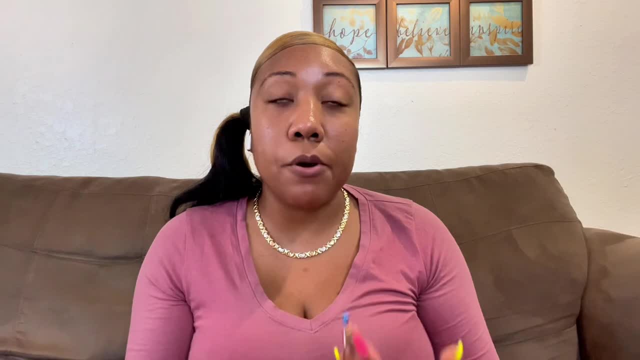 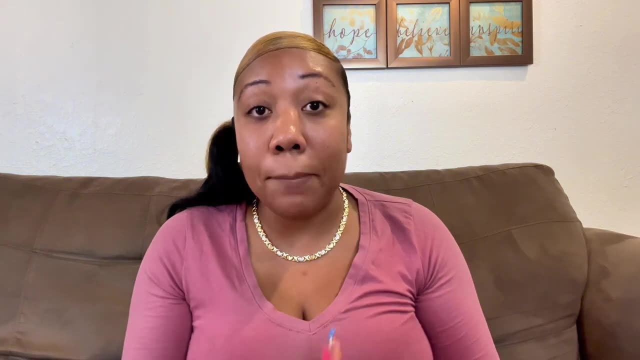 you'll know that you'll meet that person again someday. you know you can feel that person's spirit within you. um, that person's still around. it will not fix the issue. it cannot bring the person back, but it will help you to better be able to cope with it. there's also grieving courses. 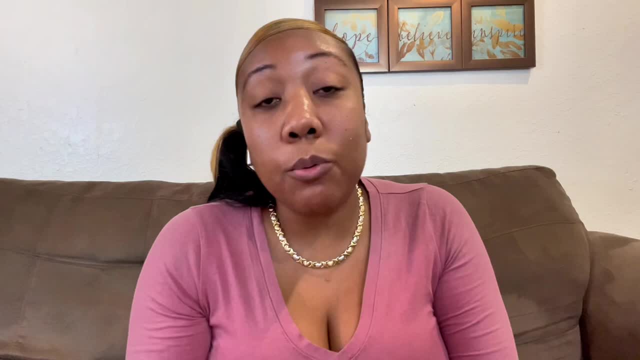 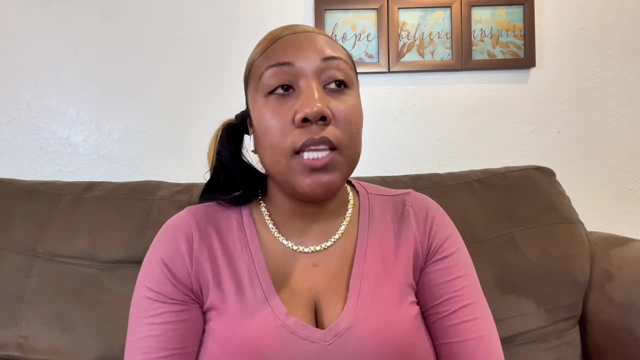 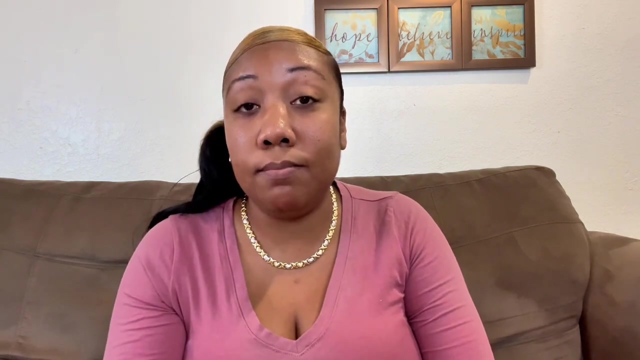 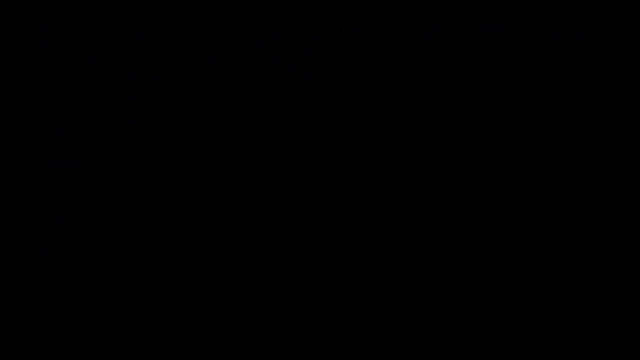 and different things that you can do to be able to cope with grief, always find a solution to your problems. if there's absolutely no way that you can come up with a solution, then you have to change the way that you view it. and if you change the way that you view things, then that is still a solution. good day y'all.